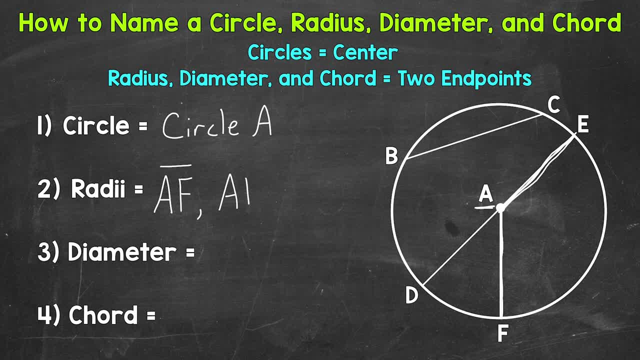 We name this by the endpoints, So A, E, and then put the line segment symbol above our two endpoints And then the last radius example here would be the center to point D here. So let's write our two endpoints, A and D, and then the line segment symbol above those two endpoints. 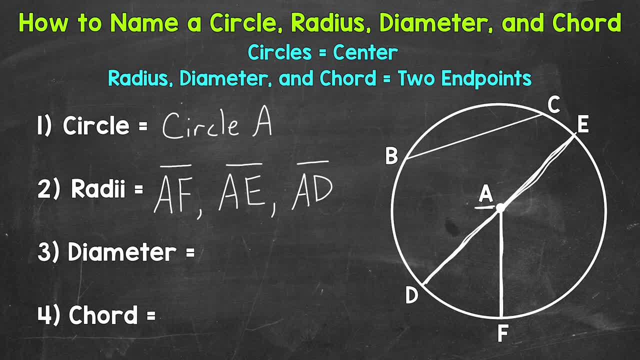 Now one more thing to keep in mind about the radius. Remember to write our point E to show another example of a radius, even though the line segment symbol is not the same as the endpoints. So let's add a little bit of center and then put the line segment symbol into our example. 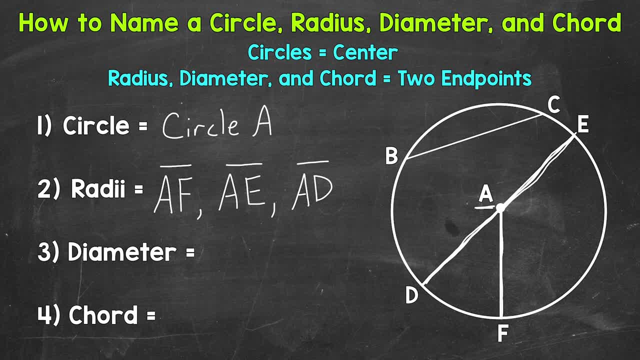 So again, let's write our point E to show another example of C. So we need to add two endpoints to the endpoints and put the line segment symbol above the center of our circle, So that way we can see that we've all connected. 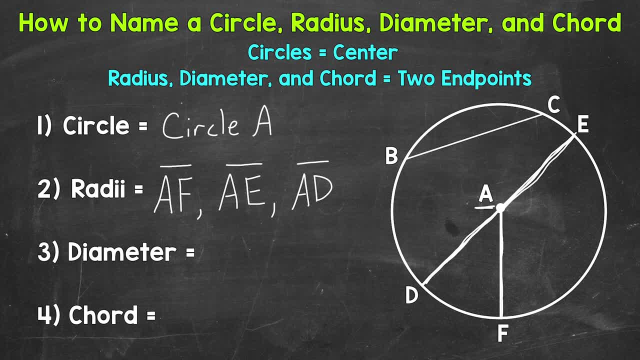 We've all joined together. See, The diameter of our example is right here. So point D goes through the center all the way to point E. So those two radii together equal that diameter. So we use the two endpoints D and E and put the line segment symbol above it. 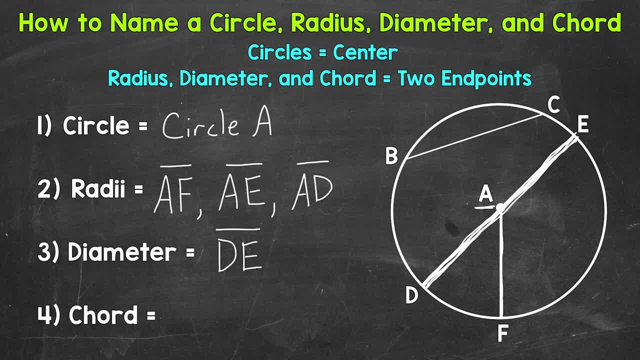 So that tells us that we start at point D and our line segment goes over to point E. Now you may be thinking that we used our diameter to name two of our radii, And that's true. A diameter is twice the length of a radius, or vice versa. 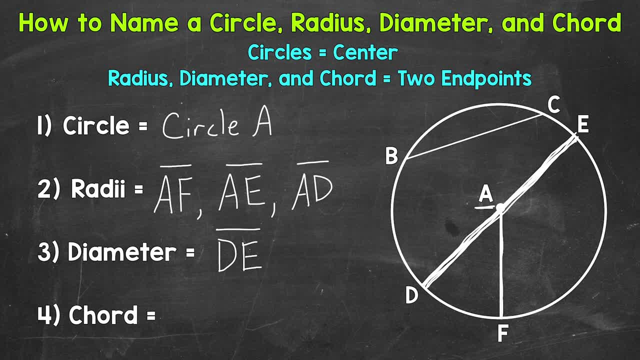 A radius is half a diameter, So two of our radii create the diameter, And when it comes to naming a radius and a diameter, endpoints are so important because they tell us exactly what line segment we should be looking at and where it starts and ends. 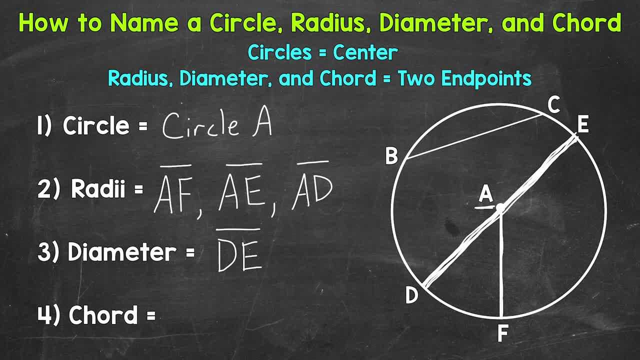 Lastly, let's name a chord And remember: a chord is a line segment that connects two points on the circle. A diameter is a very specific chord that has to go through the center, but a regular chord does not Just any two points on the circle.